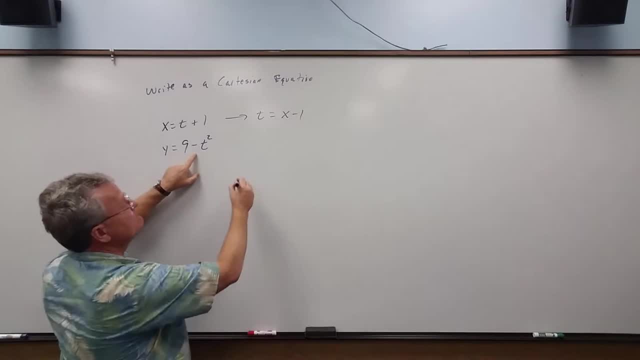 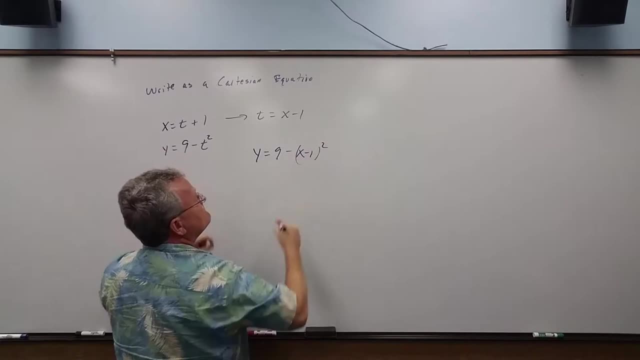 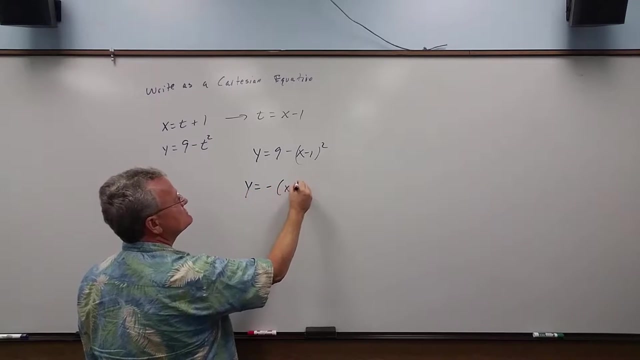 Now we substitute that into this other equation and we get: y is equal to 9 minus t squared, but t is x minus 1.. All right, So what we have here, let me just rewrite this. Let's write this as minus x minus 1, squared plus 9.. 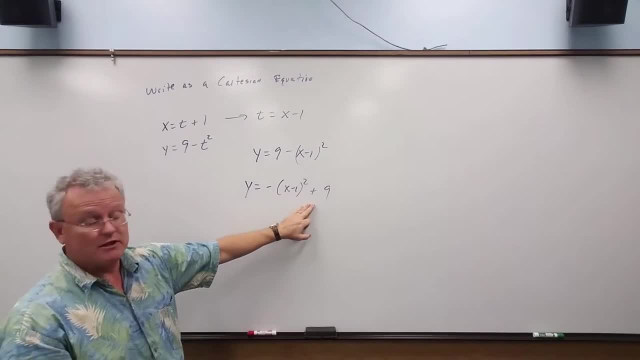 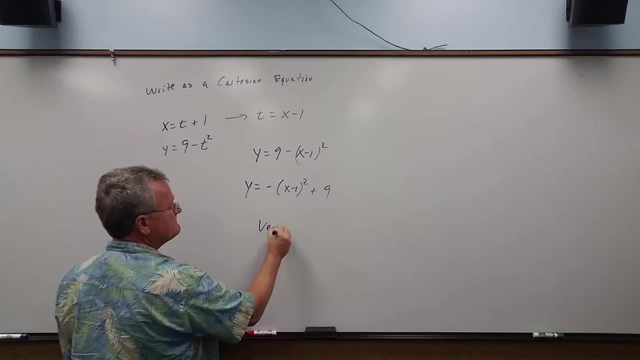 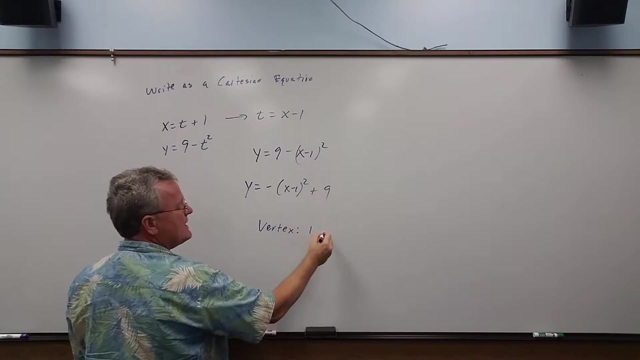 We know the graph of this is a parabola. We studied this in algebra, So this is a parabola. We know the vertex is the point h, k. h is 1, k is positive 9.. We also have a parabola. 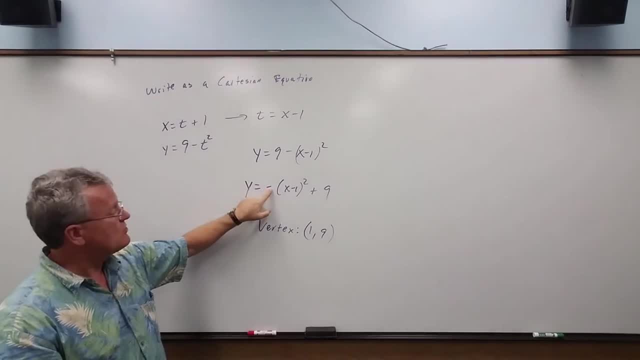 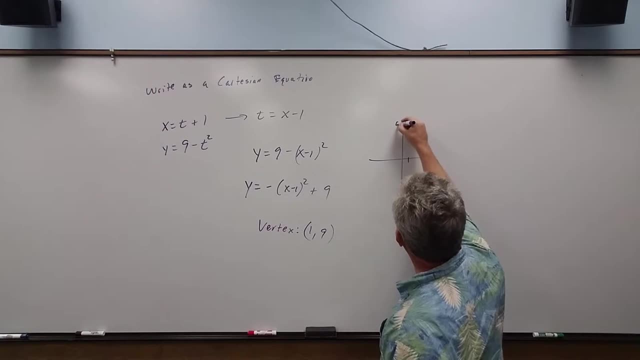 We also have a parabola. We also know it's going to open upside down because of the negative coefficient of the square. So we know it's going to look something like this: x is 1, y is up here at 9, and it's going to kind of go like this: 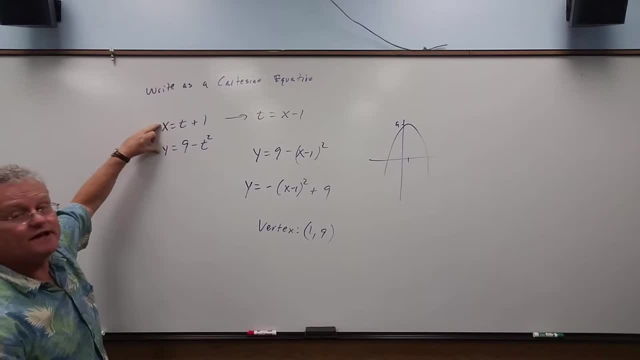 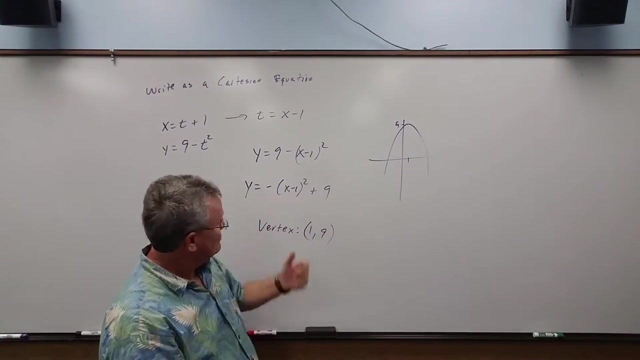 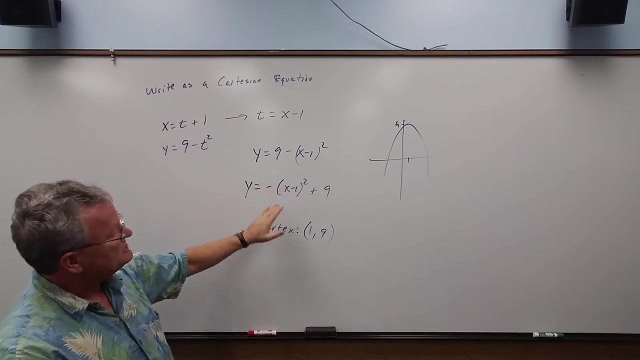 Now what's the advantage of having this? We're going to graph this in the next video, But what's the advantage to having a parametric equation instead of a of a graph given in Cartesian? in a Cartesian equation, The difference is. in a Cartesian equation, we've just got a graph. It's this upside-down parabola. 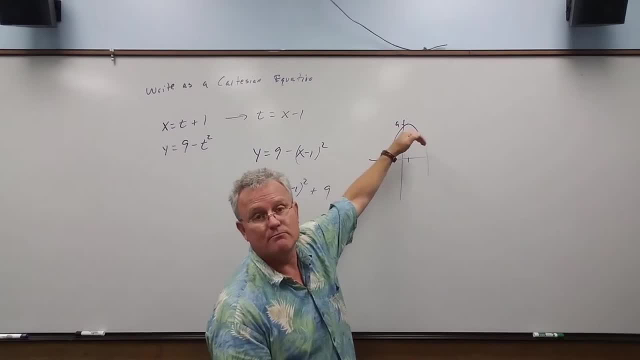 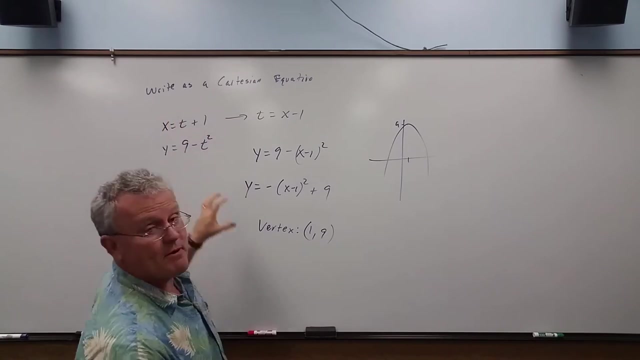 This tells us the direction we're moving along the curve. That's called the orientation. So it's the direction we're moving along the curve, And if t represents time, then I can figure out if this is where a particle is located at any point in time. 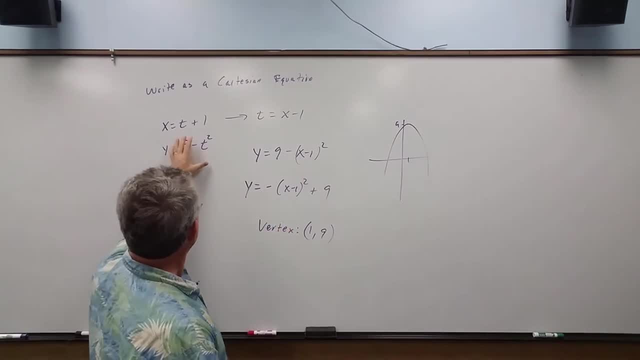 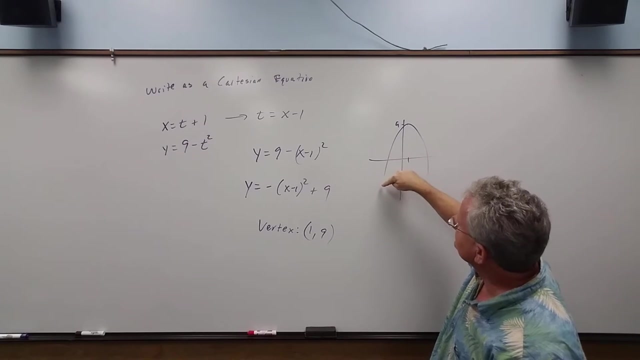 then I can plug in my point in time and I can figure out exactly where a particle is located at any point in time. So the nice thing: Here we just got a graph. Here we're going to get the same graph, but it's going to tell us the direction we're moving along the graph.